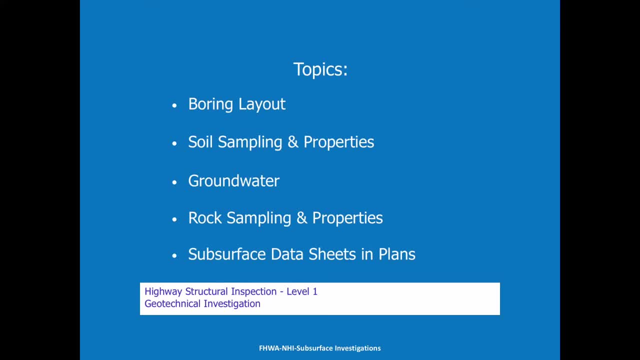 where is it? what is it? how does it affect our job, rock sampling and properties? and then the subsurface data sheets in the plans, and how do we use those and what is your role with those as the inspector? So boring layout. we'll get started So you'll see first few sheets. 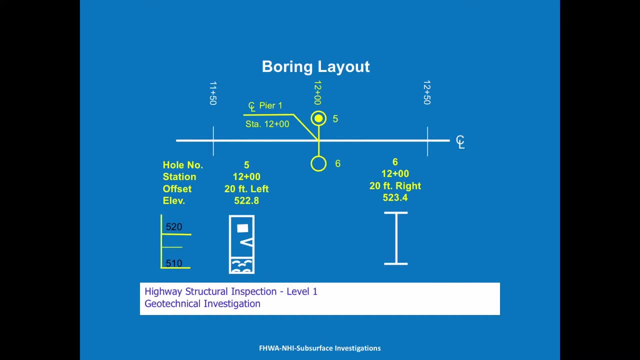 usually S4 or so. your bridge plans will be your boring layout. it'll give you center line of bridge with stations and then at each substructure location so invent or abutment pier one, pier two, so on. they'll show those on the boring layout. typically they'll do borings or auger refusals at every substructure. 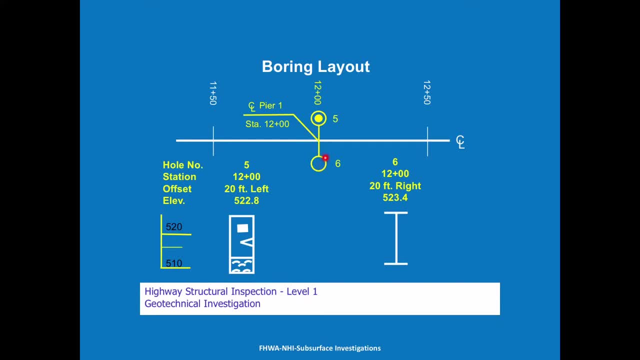 unit here. we did two at pier. number one, an open circle is just a refusal. a shaded in circle inside a larger circle is a core hole and here you can see this is core hole number five. if you go down here to hole station number five, it gives you all the information. it's at station twelve plus not. 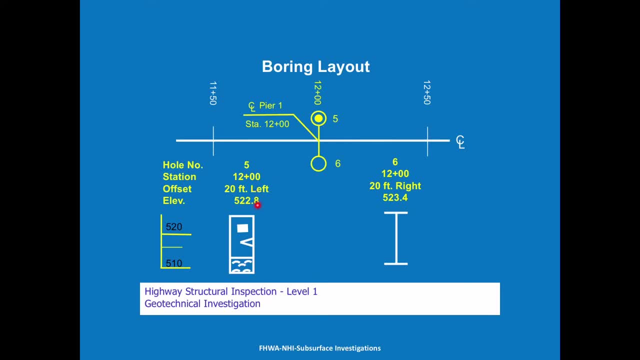 not. it was taken twenty foot left of center line. the elevation of ground line when they drilled was five, twenty two point eight, eight or eight, and then you see what type of soil it was. we'll talk more about that later. but at six it was just a boring to refusal and as you see that here, 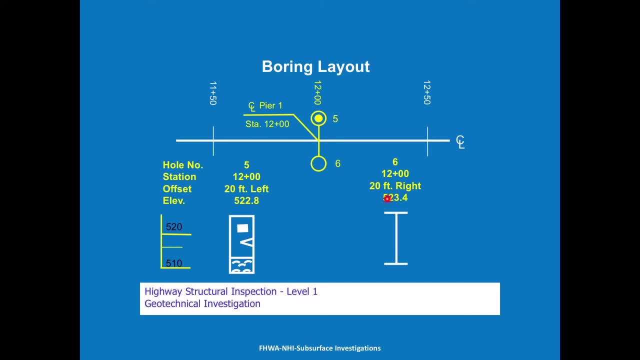 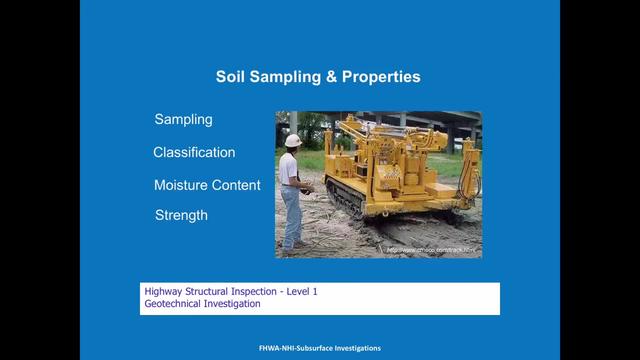 same information. twelve, now twenty- foot right had a different starting elevation, but there would be a refusal elevation down here. so why do we take soil samples? we need to sample it to be able to classify it. our designers need to know what's there to know how to design the bridge. as the inspector, you need to know what's. 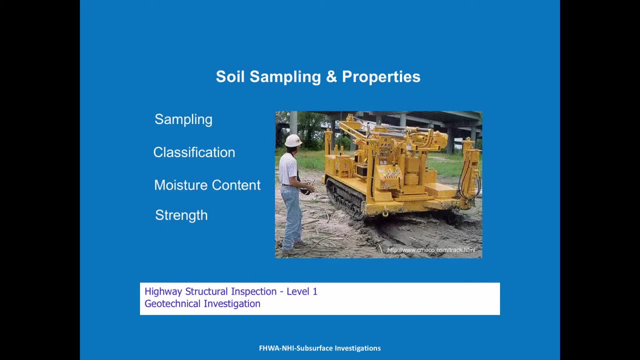 there. to know how to come use this soil to backfill the bridge, you need to know what the moisture content- especially the contractor needs to know what the moisture content is to whether or not they'll need a cofferdam or shoring. we'll need to monitor content if you're doing backfill with. 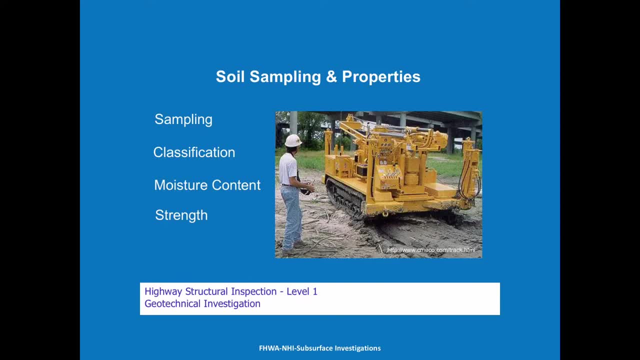 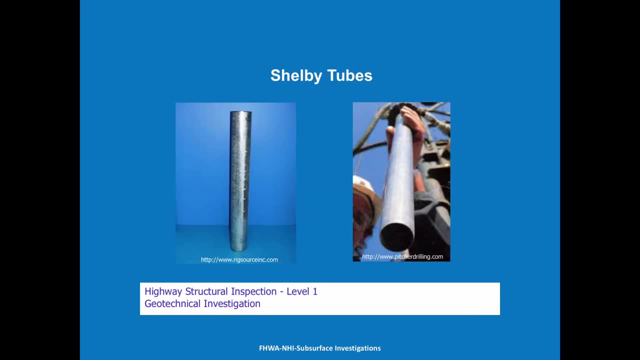 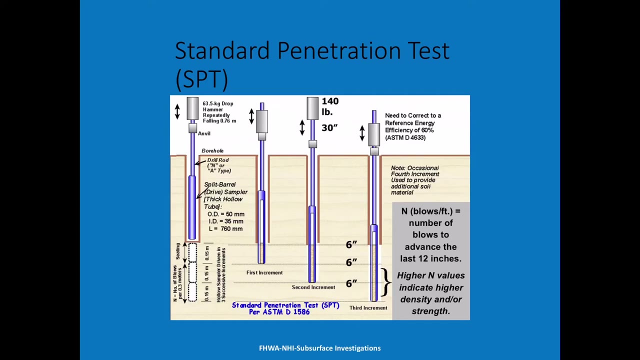 soil and then also the strength. what is it going to do when we backfill with it? we get soil samples by shelby tubes. we drive the tubes in the ground to get our sample. also, we have the standard penetration test. we drive a rod down into the ground with a set weighted hammer with a set. 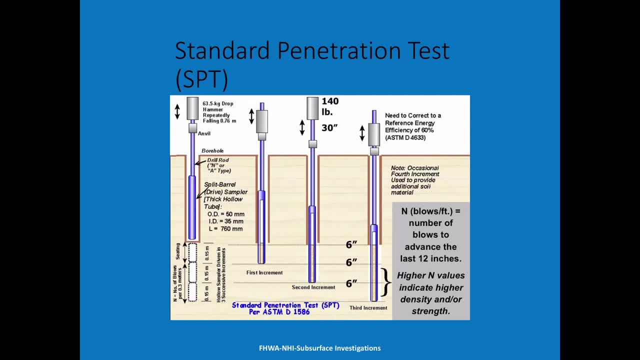 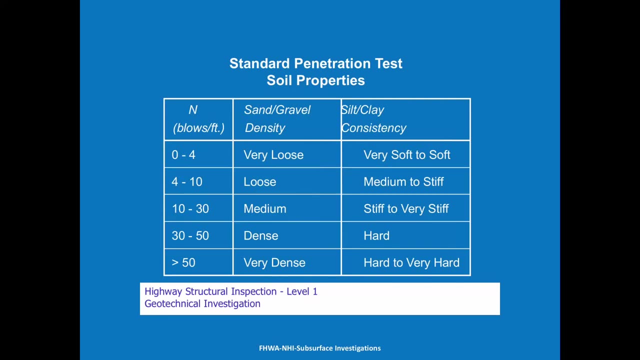 fall on it and we record the number of blows that it takes to advance the last 12 inches. so, and then we record those as an n value on your plans. so if you look what that n value represents, so n blows per foot of zero to four is a very loose if you're in a sand and gravel or if you're. 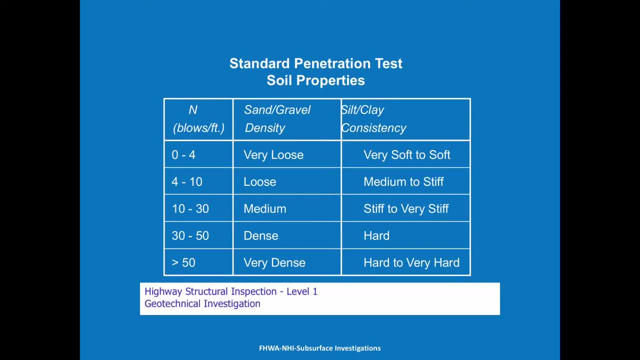 in silt and clay, a soft to a very soft. if you move down to, we'll say, a n value of 10 to 30, you're in a medium density sanding gravel or a stiff to very stiff silt and clay. so these will kind of help you. 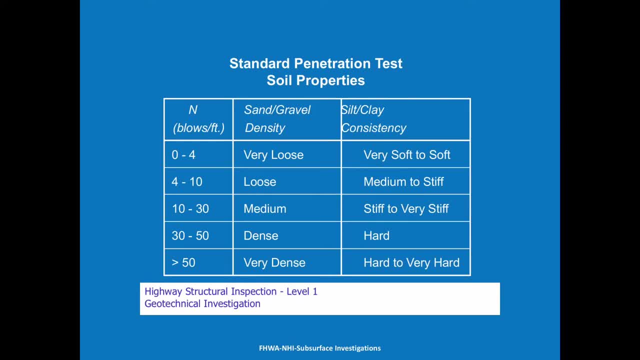 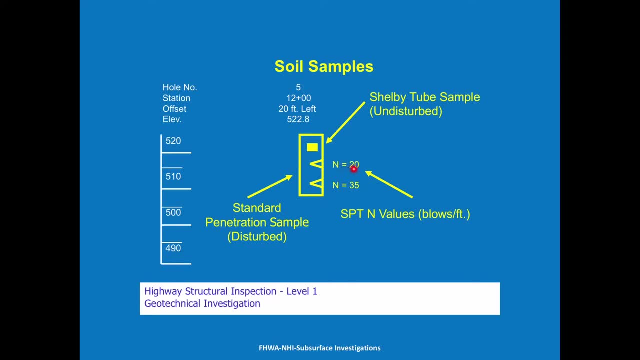 with the해도ing, the soil, and then a lot of this material, however, is a very high rag, might be different if you were in a sand or gravel, or so do what type of material you're working with. you can see here, outside the core sample. the n value at this elevation is at 25 feet down at 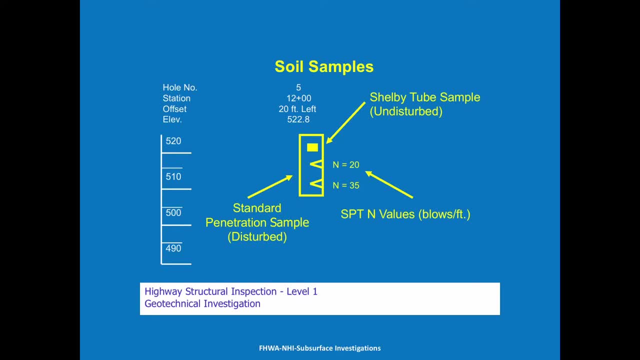 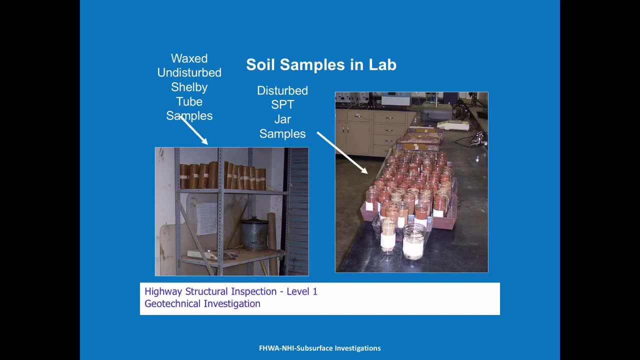 the elevation. it's 35. it's telling you we're more and more dense soil the further down you go. here's what the samples look like in the lab before we test them. you've got some waxed, undisturbed shelby tube samples and then some disturbed shelby tubes, and then we give them the first bunch of and we've show again what's happening here is, when you're using the n value, the sample, it's getting a completely different sample. now we're going to do it like this and i'll add the sample sample into the sample sample and then we'll go ahead, and we'll go ahead and we'll put some more there, and we'll put some more. 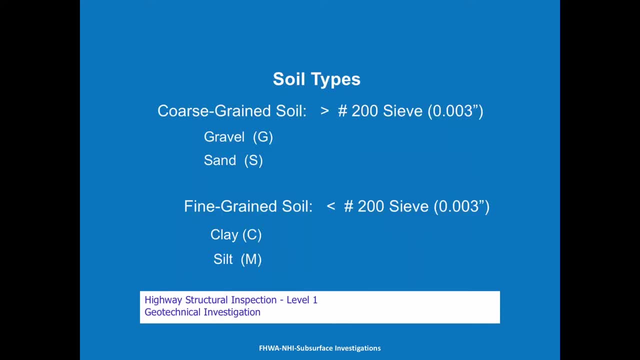 SPT jar samples. all right, so what are our soil types? if you look at the unified system, you got the unified and AASHTO we're gonna cover unified here. you can look more up that later on other videos or just kind of look on some. 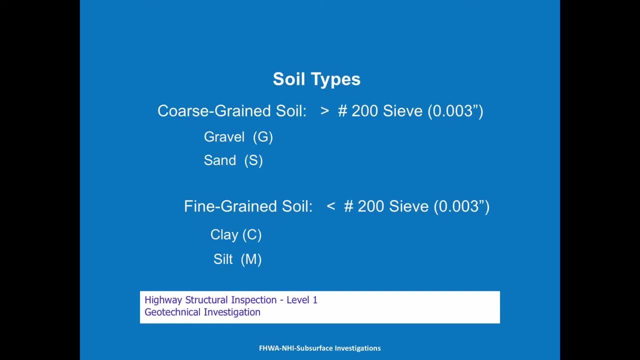 AASHTO different classification websites, coarse-grained soils or any soils that are retained on a number 200 sieve. that new number 200 sieve is that magic sieve. it can actually hold water, but so anything above that's our gravels and our sands. anything that passes through that number 200 sieve is our fine-grained. 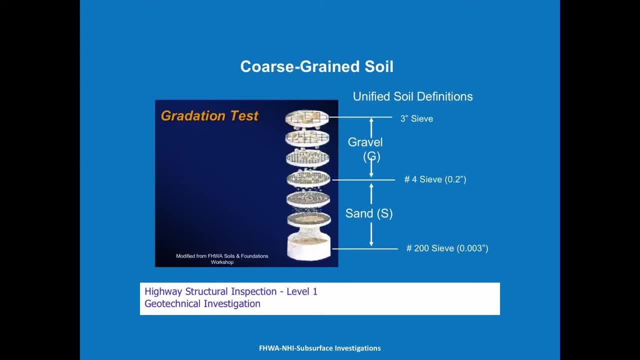 soils of clay or silts. so this is our sieve analysis. as you can see, anything from a number four and up is considered a gravel and anything from the number four and down is considered a sand, and then anything goes below the 200 sieve is a silt or a clay. 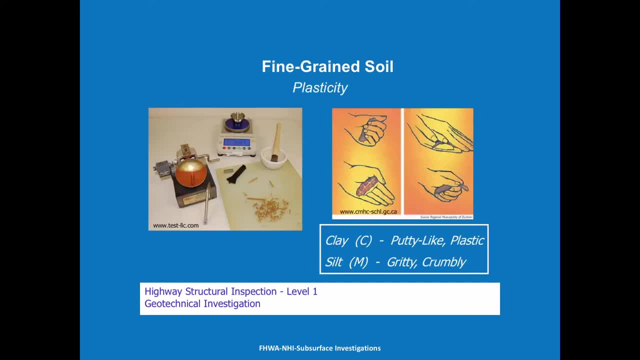 two different types of sieves that we're going to cover in this video are the two different types of sieves that we're going to cover in this video? are the determined the difference in the silt and clay? we know silts are more gritty, clays are more putty like, but we can run different tests. you can see a picture. 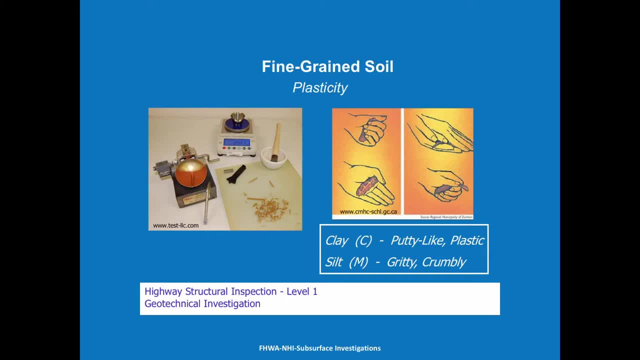 here of the Atterberg limits test and just doing a test in our hands, rolling it together to be able to determine do we have a clay, do we have a silt? and there's more tests that can be run in the lab to determine actual percentages. 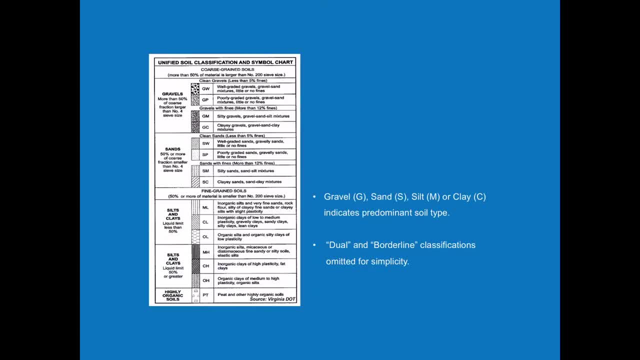 using a hydrometer and such. so here is a picture of the unified soil classification system chart. it would be good to know this because you know what these initials are. so: GWG, GP, GM, GC- the GW is a gravel and it's well graded. you can see here: well graded. 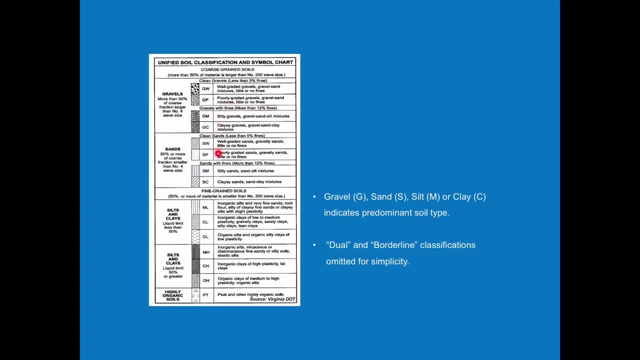 gravels P is a poorly graded. so the same goes for sand- well graded, poorly graded. you down in silts and clays, you're going to see L's and H's. that's low plasticity, high plasticity. if you need to know more about this, take our grade and drain. 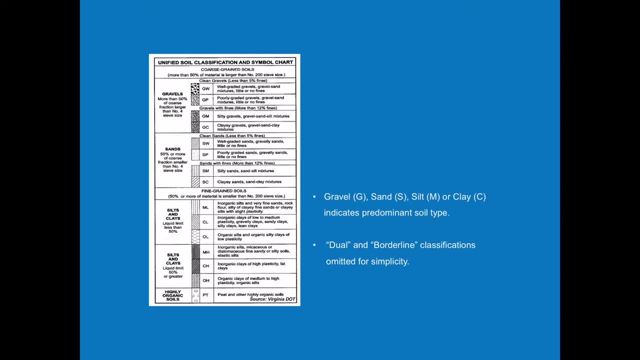 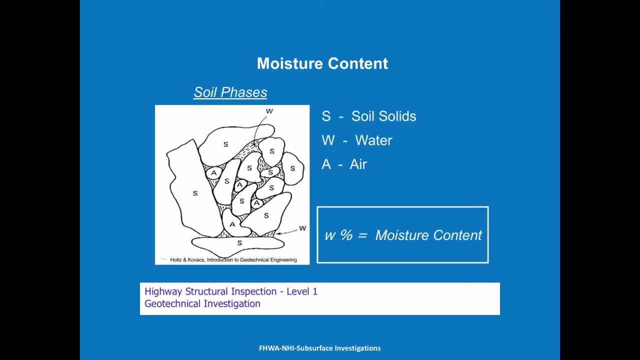 class that we offer. this class goes way more into depth into this and is actually a prerequisite for our class, for this class in person. so if you look what is moisture content, if you can see here this diagram, we've got the s's label: soil, the little bubbles with a's. 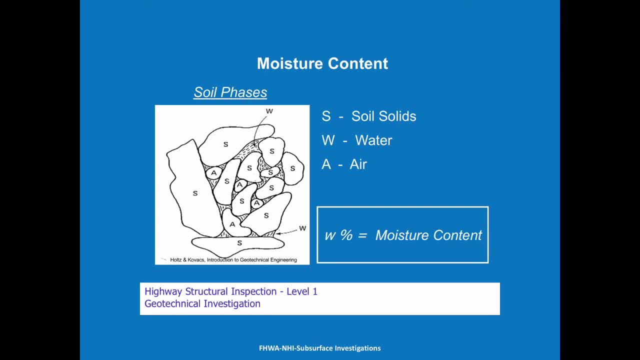 or air, and then everything in between is water, so we can weigh it dry it. weigh it dry and we get that moisture content. how much water is actually in the soil? water is a good thing in soil, but it's also a bad thing if you have too little it. 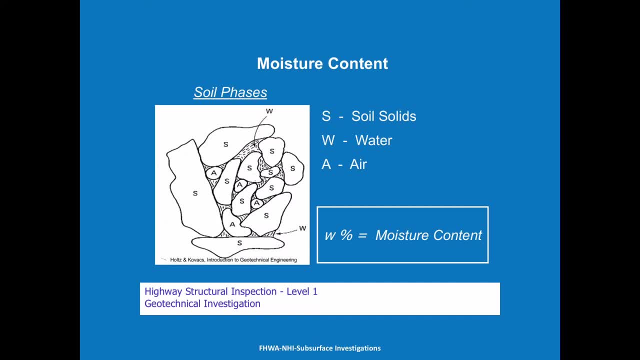 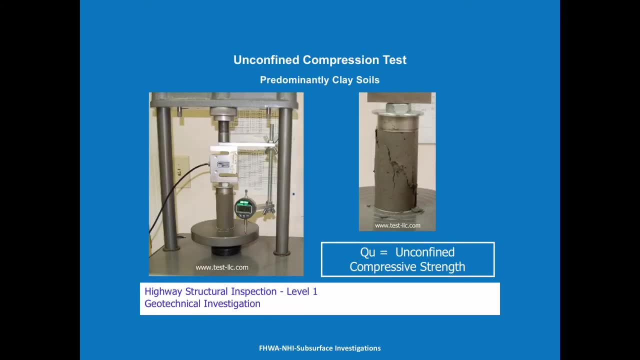 won't act right. if you have too much, it won't act right, but if you have just enough, it'll do exactly what it's supposed to do. it can give you the compaction to do your work. the unconfined compression test gives us a strength of our soil, just like we get a compressive strength. 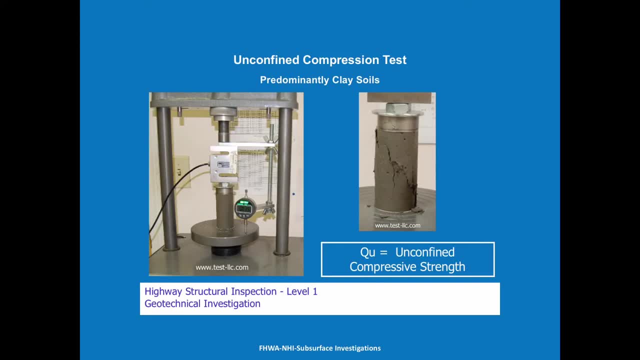 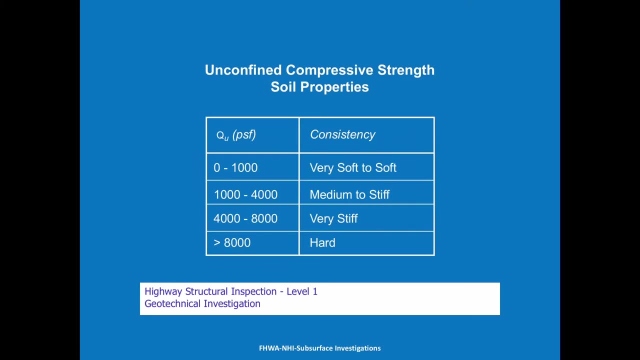 of concrete we can get a compressive strength of this soil, so we mold it together in a cylinder and then you break it. very similar but as you'll notice, we got different values. a medium to stiff is a thousand to four thousand and you think four thousand that's pretty more than stiff on concrete. 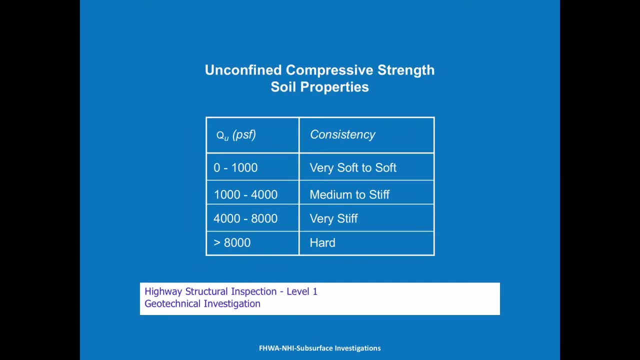 well, on concrete that's 4,000 psi. on soil that is 4,000 psf, so pounds per square foot, much larger area to give you a much different consistency and density. so here 4,000 psf is a medium, is a stiff compressive strength different than 4,000 psi in concrete. so that is a qu. 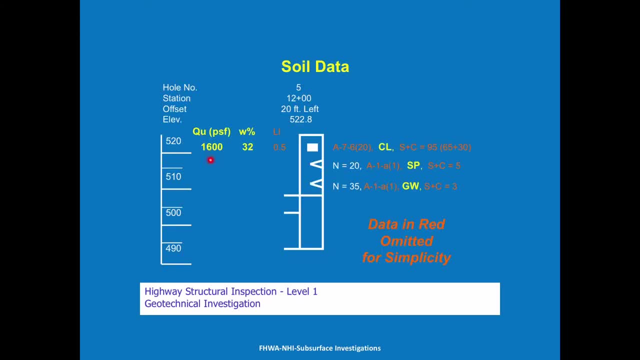 if you're looking on the plans you can see the qu is going to be right outside. here it's to give us and this test. it's a 1600 PSF and has a 32% water. Here you can see CL if we. 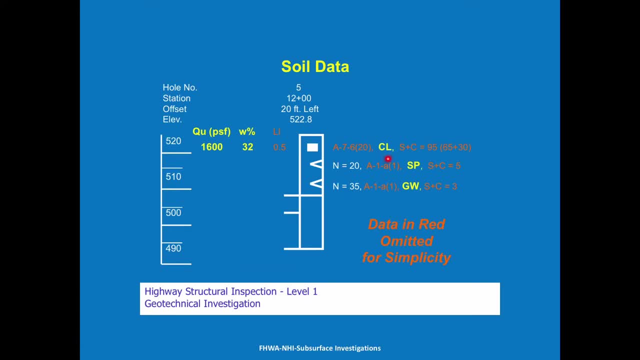 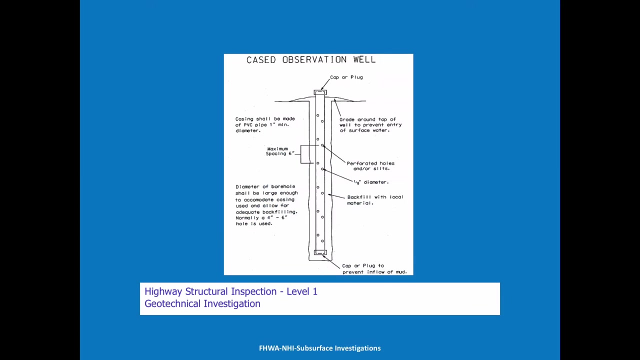 remember back to our chart. that is a clay with a low plasticity. Here we have a sand that is poorly graded and a G that is well graded. Our end value here is 35,. our end value here is 20.. A cased observation. well, is what we're going to. 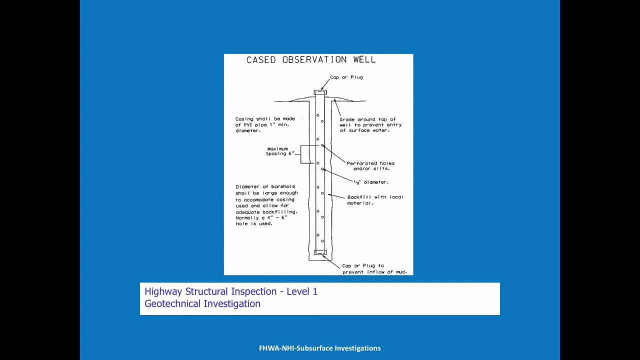 use to know where the water level is. So when they drill down for refusal, on just an auger drilling, they're going to pull one of these observation wells and then we'll measure where is the water table and check it over time to see how it. 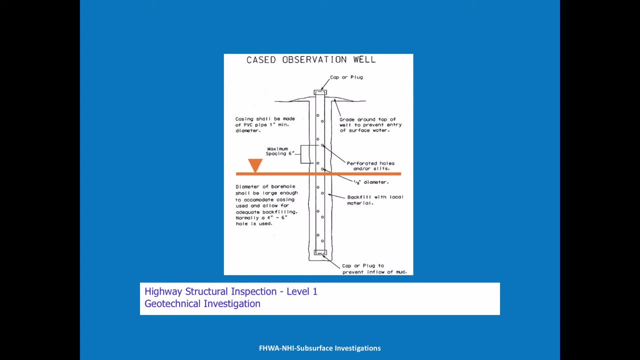 fluctuates. The contractor needs to know this to know: do I need a cofferdam? do I need extra shoring? what am I going to do to protect this excavation until I get my concrete poured and backfilled? So our rock sounding an observation, well so. 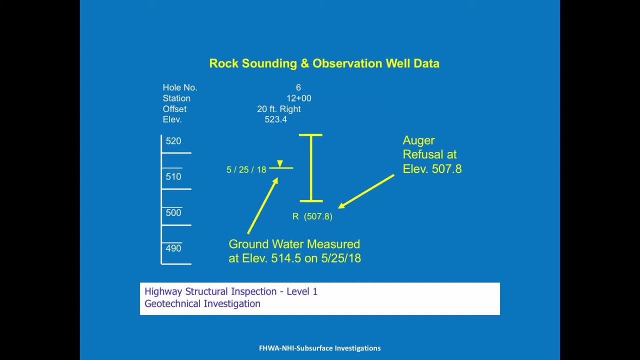 we're moving now from soil to rock sounding. Rock sounding here. we've got a similar thing You've got in this instance, just a refusal. Our auger refused at 507.. We've drilled down and we've got the date. so that way the contractor knows, probably in the wet. 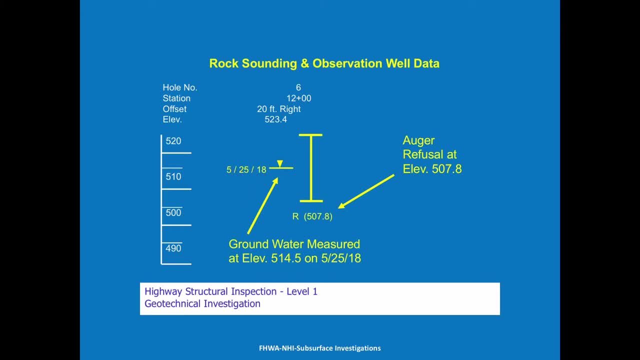 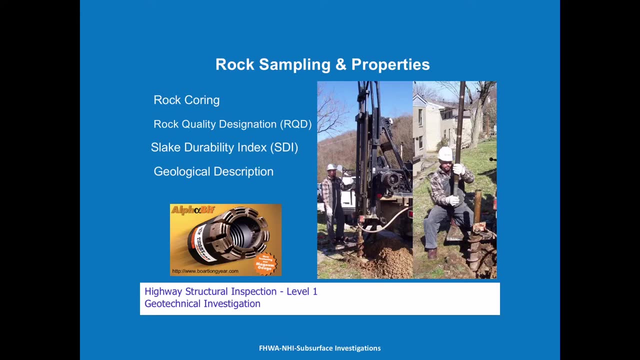 season We get more in June. July. that's going to lower as it dries out. Now, rock sampling and properties: With this section we're going to talk on rock coring, the rock quality, and then we're going to talk a little bit about the. 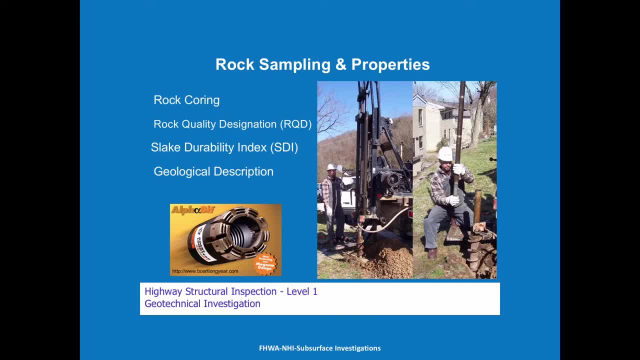 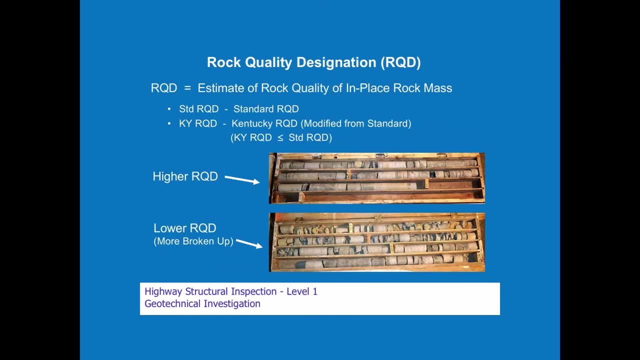 quality designation of the RQD and the Kentucky RQD, the slake durability index, and the geological description. So RQD, or rock quality designation, is the estimate of rock quality, of in-place rock mass. From what I understand it that: 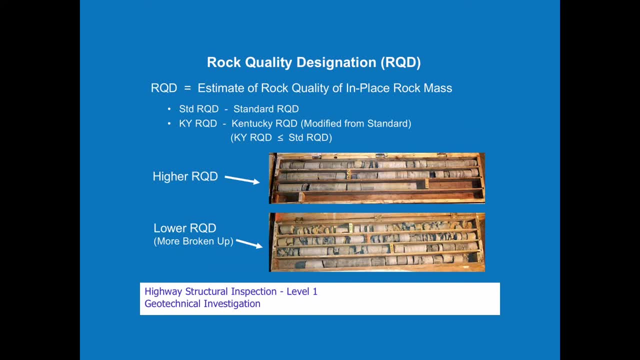 is sections that are four inches or larger get counted and gets a percentage of the total run of five feet. Kentucky RQD is we go in and we actually break those apart. Some of our shales we can break by hand and we don't want to. 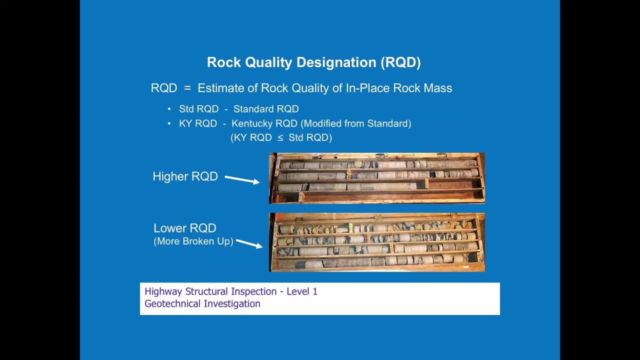 give those a high RQD count, but they will hold together in the drilling, So we break them apart. The Kentucky RQD will be less than the standard RQD because of this. You can see this first picture here. you got a higher RQD. You see a. 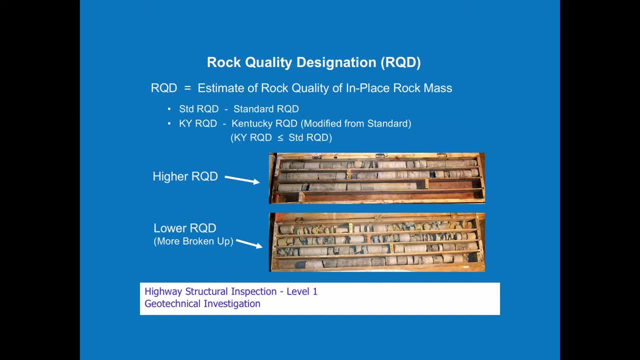 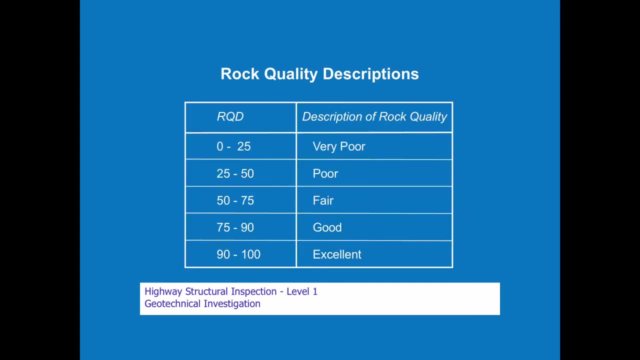 lot of the rocks together: Big long core run links, and then lower RQD is the one that's all more broken up. So our rock quality descriptions- RQD 0 to 25, is very poor and as you go increase your number. you. 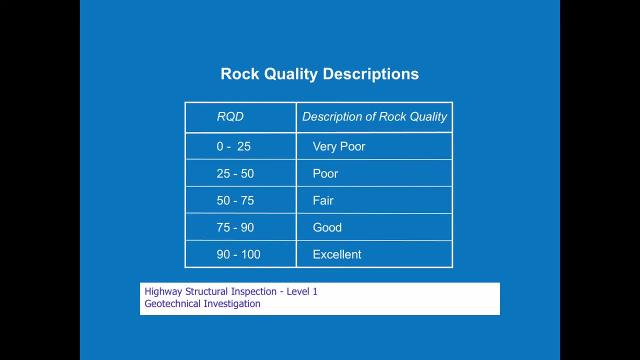 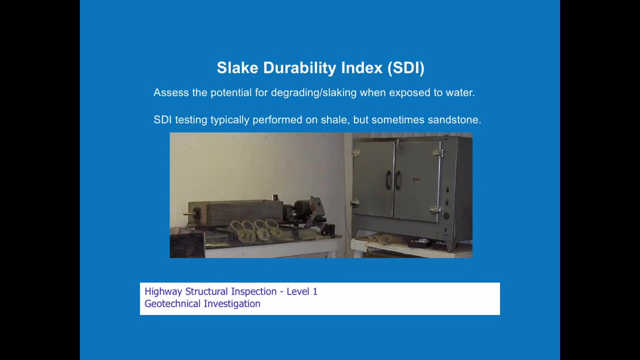 increase your quality up to excellent Alright. slaked durability index is a lab test done on shales to determine their weathering. What is the degrading and slaking when those shales are exposed to water? Some of our shales are some pretty nasty stuff that'll just fade away into. 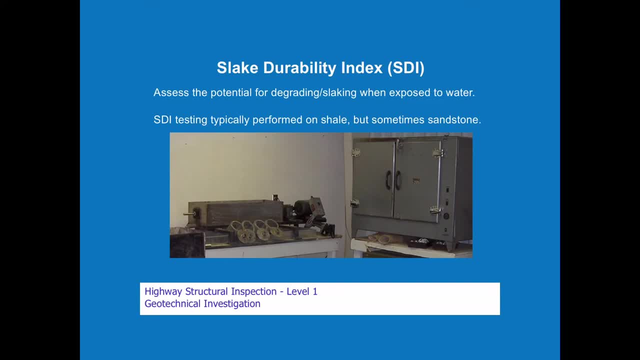 mud and almost straight water. But this is done, performed on shale, sometimes on sandstone, but mainly on shale, And we want to know what is the effect and we'll select value. So those values are 95 and up or below 95.. 95 and up, we consider a. 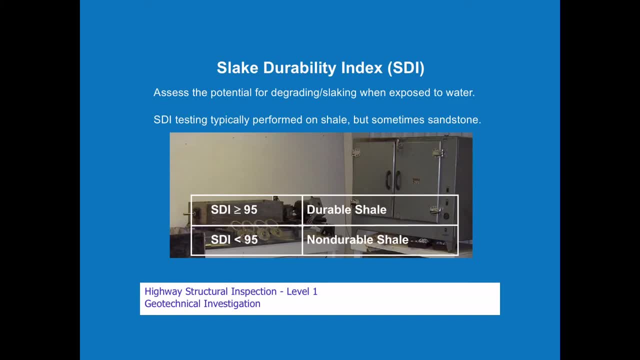 durable shale. This is a good hard rock. We have good durable shales in the state, but we have a lot more non durable shales in the state. These non durable shales, we need to know how to waste them If we are gonna use them in our fills or 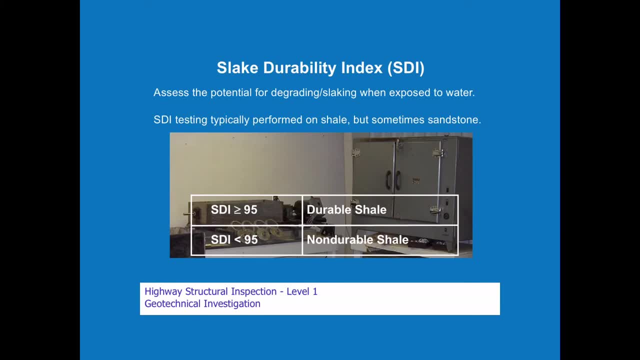 bridge back fills- Not the bridge back fill, but the fill leading up to it. We need to know what we need to do to it to make sure it's already slaked out before we start loading even more. we start loading even more on top of it. so if we're looking at our SDI values, you'll see here. 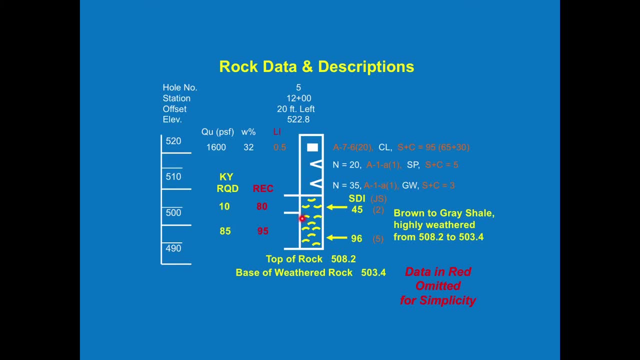 the shale is denoted with frowny faces and smiley faces. this is an SDI of 45, so we know that's a non-durable shale. non-durable shales are denoted with this frowny face. also note the Kentucky RQD. 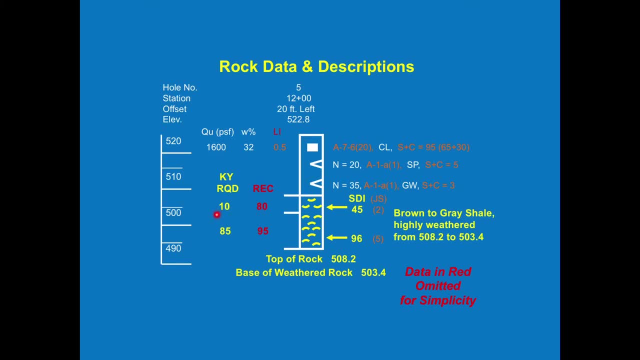 is 10, much less than the recovery, because we broke it up. it's a bad shale that breaks apart. you get further down the hole. we got an SDI of 96. that's a durable shale, denoted by the frowny face with RQD closer to the recovery- 85 and 95. so this is a much stiffer, harder shale. notice this JS here. 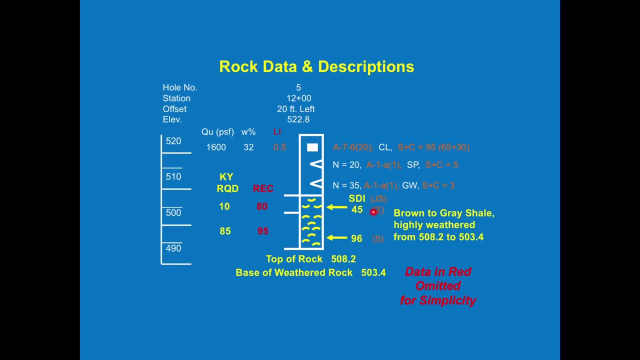 of two and five. this is called the jar slake test. it's a very subjective test of a rating one through five. you can do this. just stick a sample in a bucket in your truck and you can do a test on the shale right there to see what you have. 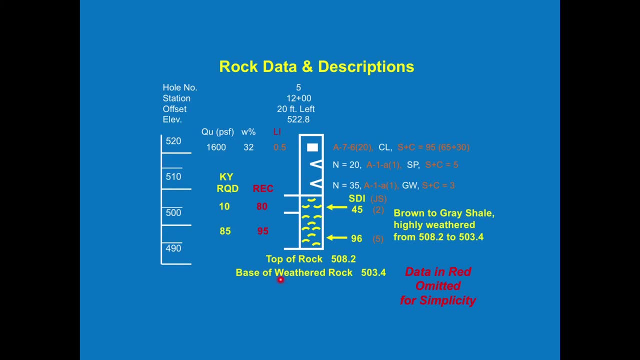 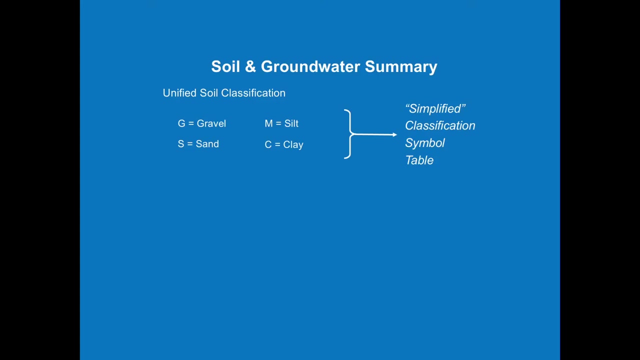 you note, here we also have top of rock and in the base, of weathered rock. that's what we're going to for our structure excavation, which we'll talk about in the next session. so, soil and groundwater summary. we're using the unified soil classification system for gravel, sand, silt and clays. 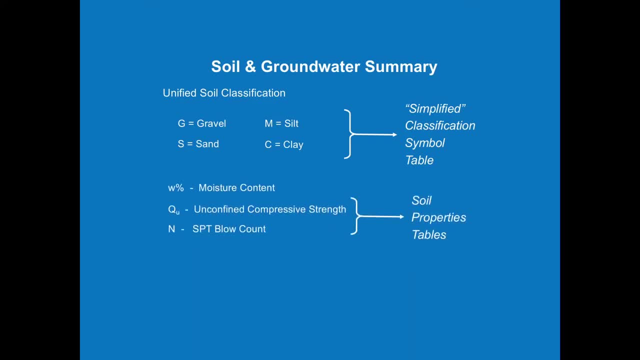 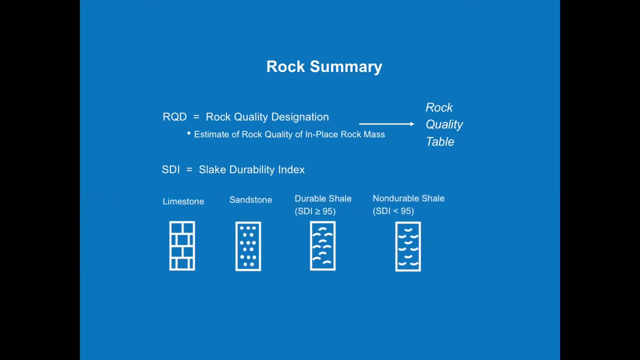 the w percents for our moisture content, our unconfined compressive strength, our n is our spt. blow count these line with the upside down triangle demarcation, widthاس, 2, Gemini, and then the number two step up and known asJason: all right can do, or fillingھی. 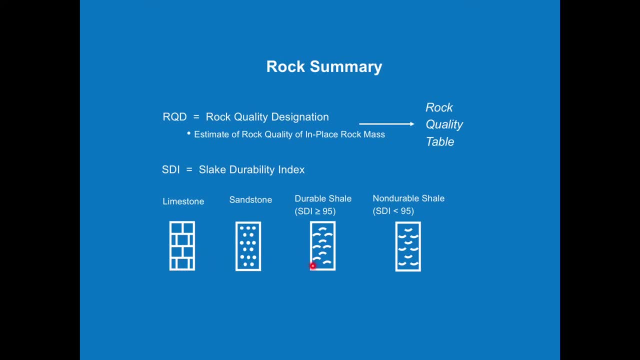 tool some options with log tirock map: forest marketplace option mark denotes groundwater table. for a rock summary, RQD is a rock quality designation. yes, minute of the rock in place, and then SDI I's are oppose. non-durable shale is denoted with smiley faces and then R would give you the. 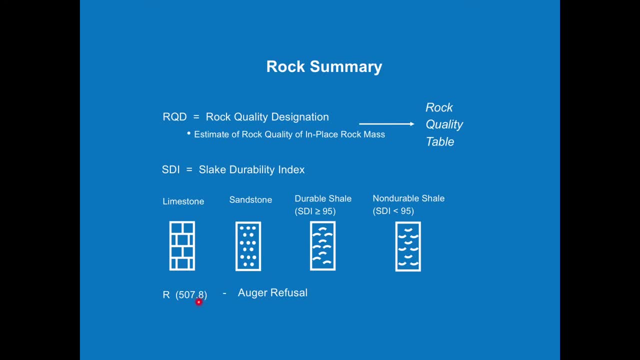 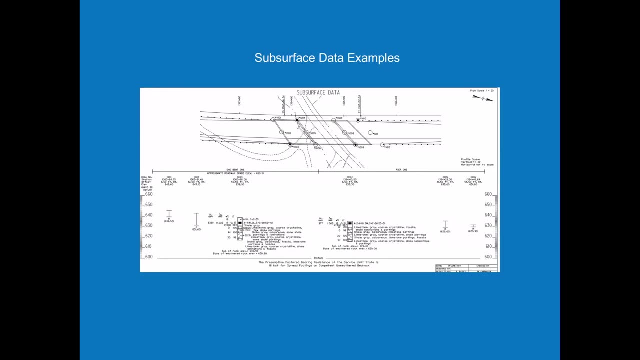 auger refusal. so we didn't take a core sample, we just drove down to rock and we stopped. so let's look an example: set of plans, full sheet. here you got the subsurface data, we've got center line of bridge, we've got all of our core hole. 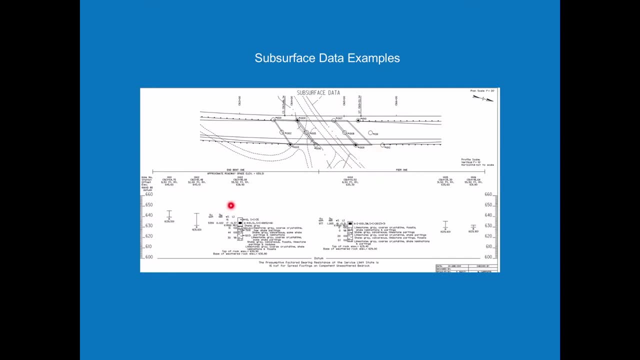 and auger refusal locations. down here you see the inbent pier, one area, and the different core numbers, the whole numbers, the station, the offset and the elevations. so here, if we look at one thousand three that comes to here, we can go straight down to look at the core data. so a zoom in of that with all the